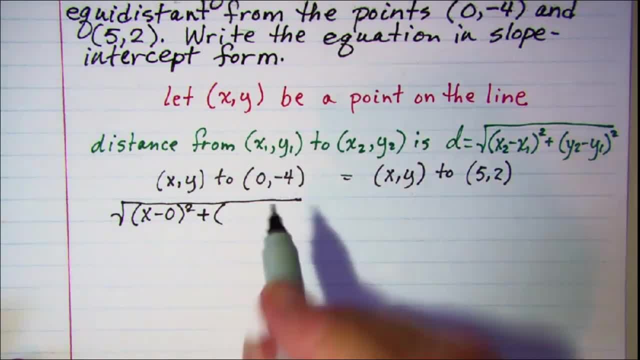 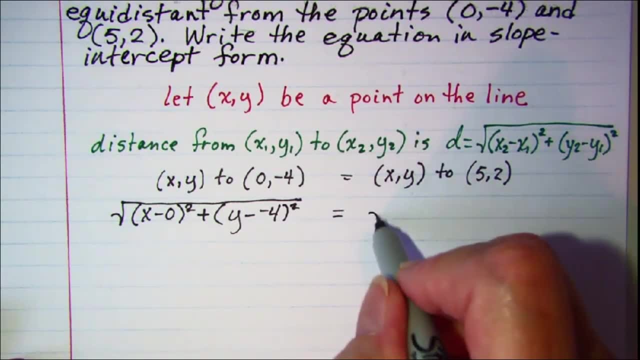 plus. And then I'm going to go with x, y subtract negative, 4, quantity squared, And that distance is equal to this distance, x subtract 5, quantity squared, and y subtract 2, quantity squared. Now, this is the equation of our line. 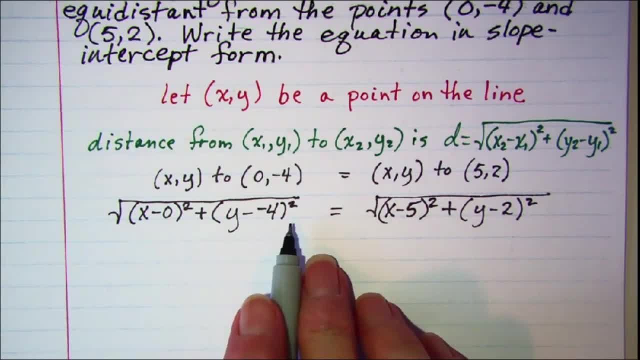 I'm going to simplify it a little bit and put it in slope-intercept form. Our first thing to do would be to remove these radicals. Please do not get creative and think that this radical removes these squares. It does not, because these squares are added together. 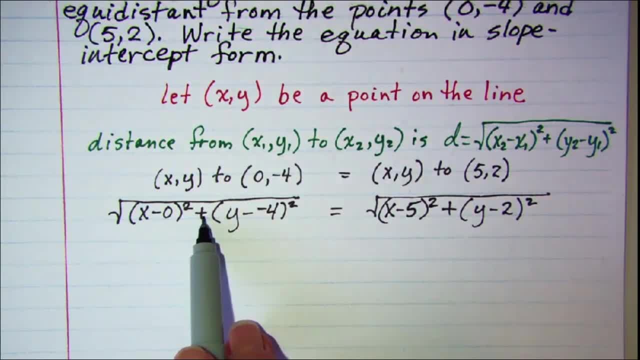 here. This is the sum, And there's no rule in mathematics that says that that square root removes those. So what we need to do, the only way to remove those radicals is to square both sides. So we'll do that first. 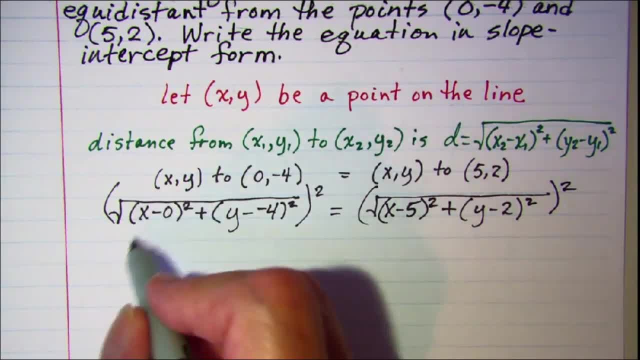 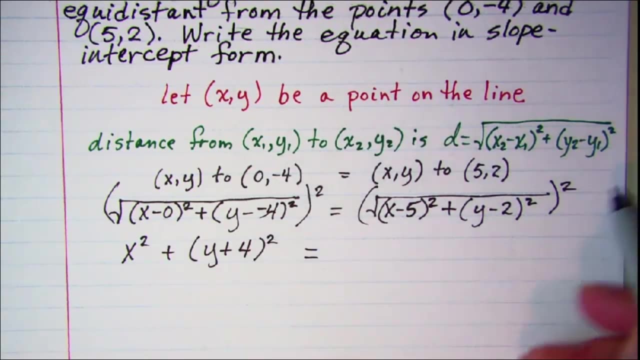 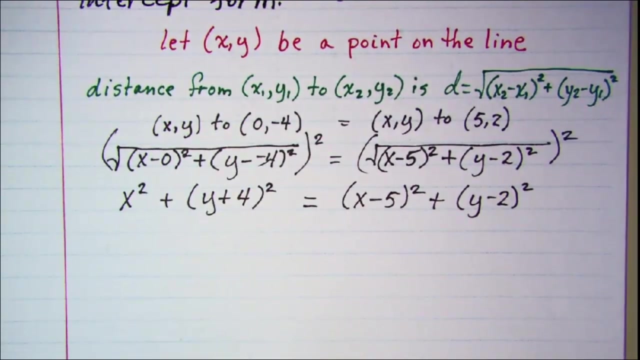 This square would remove this radical and I'll have x minus 0 squared, which is just x squared, And then y plus 4, quantity squared. And on the right side, this square removes this radical And I have x minus 5, quantity squared, and y minus 2, quantity squared. 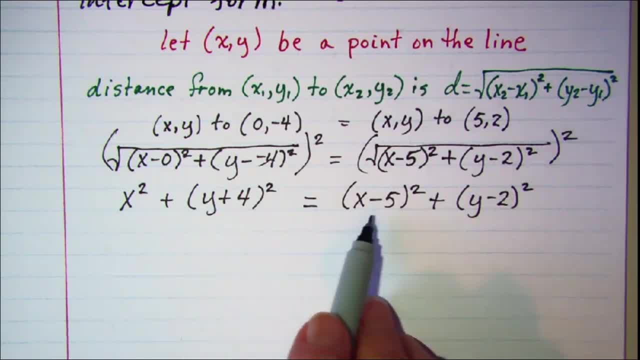 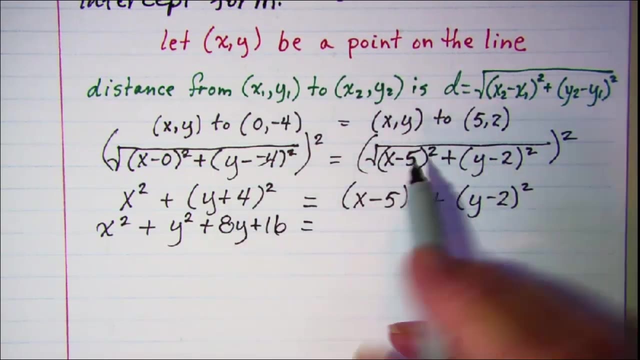 Our next step in simplifying is to square these binomials. This one's copied. And then y plus 4, quantity squared, is the same as y squared plus 8y plus 16.. And on the right side, when we square this binomial, we get x squared minus 10x plus 25.. 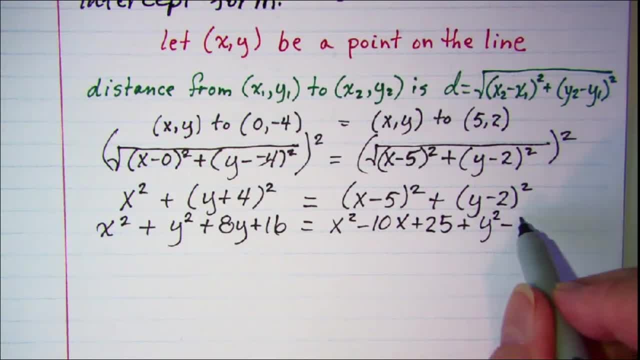 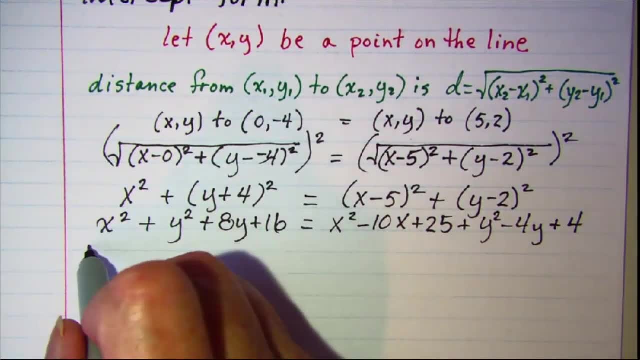 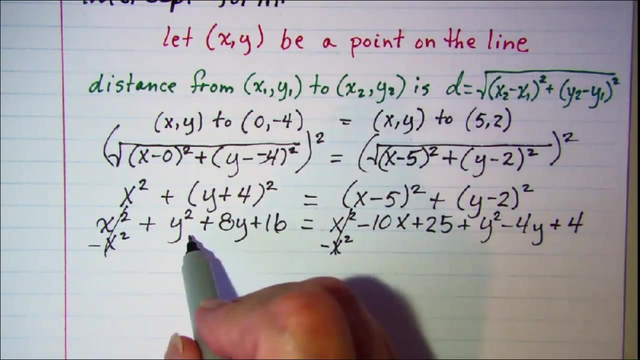 And then y squared minus 4y plus 4.. And we see that we have an x squared on both sides. so let's subtract x squared from both sides And those will cancel, And subtract y squared from both sides. Subtract, Subtract.